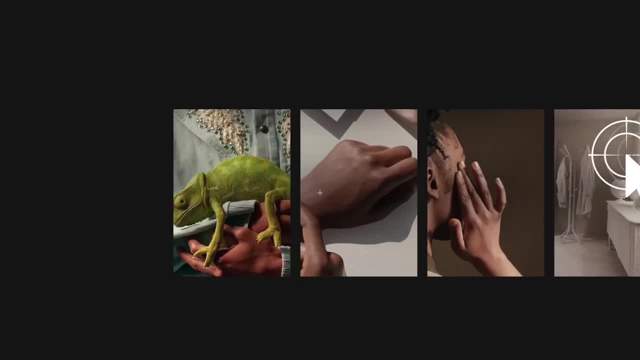 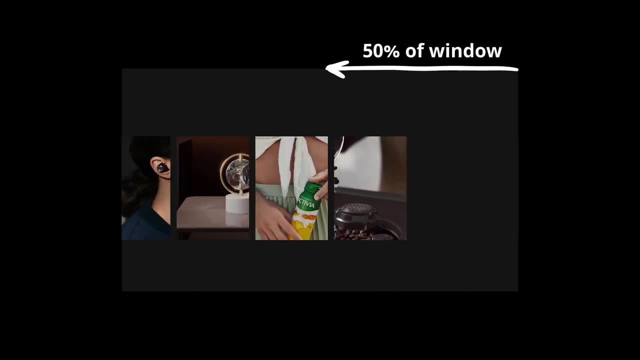 moves at a different rate of speed, So I can see how far I have to drag to get from one end of the track to the other. Aha, so by the time the mouse is halfway across the screen, the track has moved 100% of its maximum distance. So it's almost like we can imagine. there's a slider on the screen. 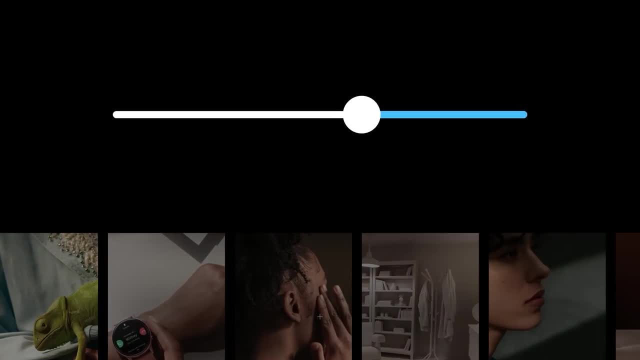 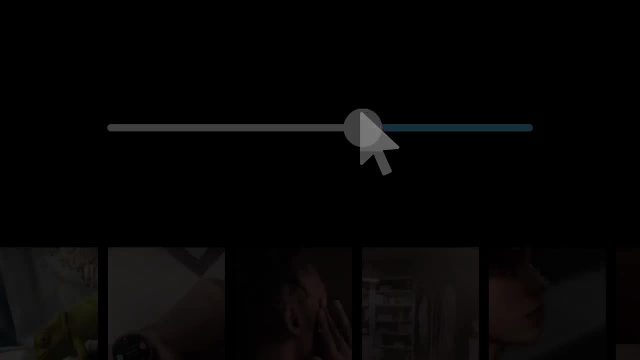 and dragging it back and forth controls our track. But this slider is extra fancy not only because it's always following our mouse around waiting for us to click and drag, but because it's completely invisible as well. So how do we go about creating our magical invisible slider? Well, the very first. 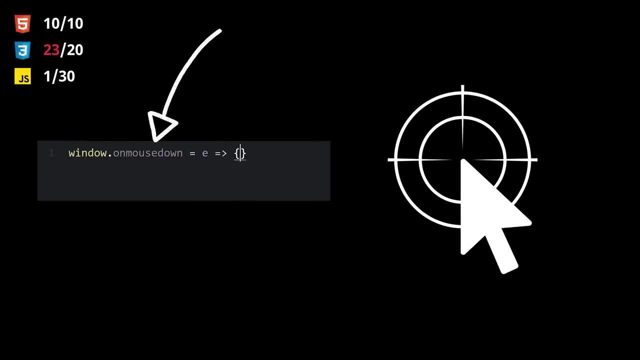 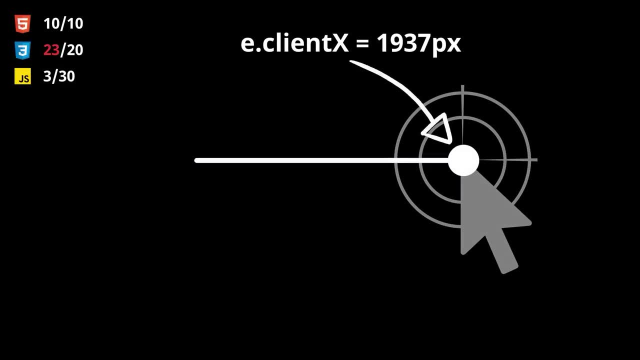 step is pressing our mouse down. So let's start by listening to any mouse down event that may occur. When that happens, I know I want to keep track of the exact X position the mouse was at so we can use that as the starting point for our invisible slider. But where are we going to store? 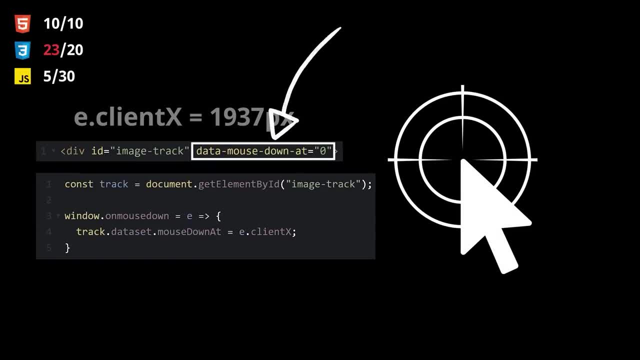 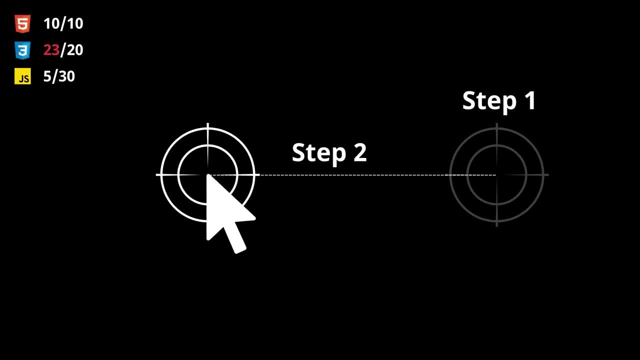 that value? What if we just created a new custom value on our track element that will update every time the mouse is pressed down? Alright, what happens next? Step 1 was mouse down. Step 2, the mouse moves. So we need a mouse move listener. We need a way to know how far our mouse has. 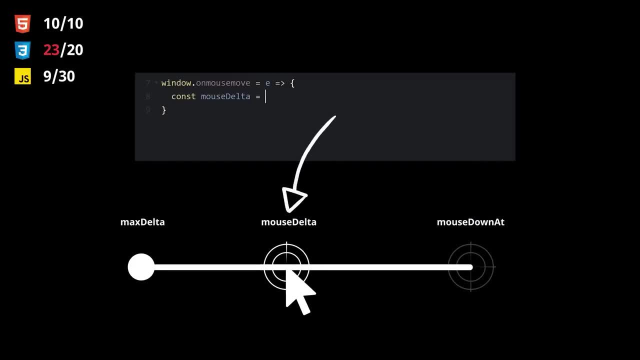 as well as where the other end of our slider should be. The relative position is easy enough. Just subtract the current position from the starting point and we already know. the max distance is one half of the width of the window. So dividing the relative position by the max, 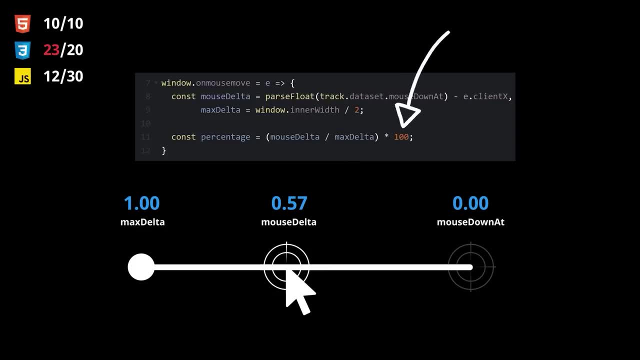 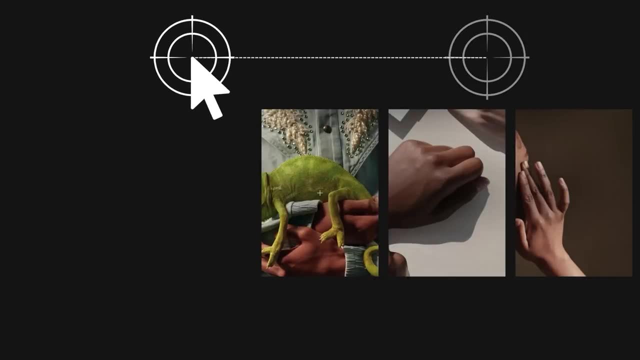 distance would convert this value to a decimal, And multiplying the decimal by 100 gives us a percentage. Oh wait, my head hurts. Why were we even doing this again? Oh right, because clicking and dragging halfway across the screen has to move our image track from one end all the way to the. 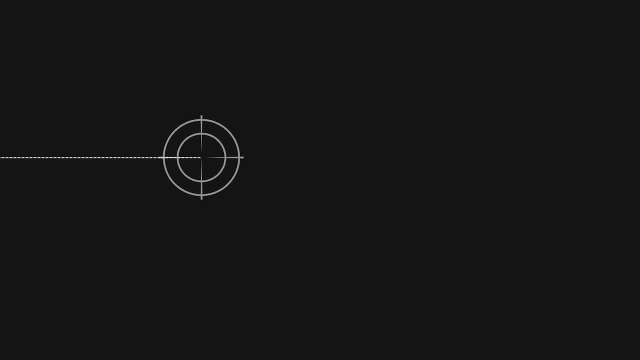 other. Only this functionality has to be possible, no matter where we click and drag. So let's click on the screen. So by tracking the starting point and using it to create a virtual slider, using math, we can thereby obtain the value we truly need, which is the percentage of our slider. 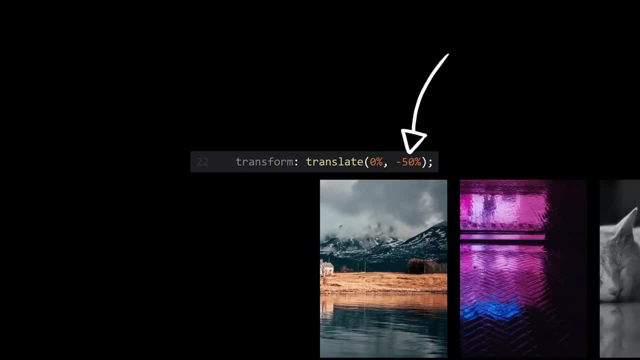 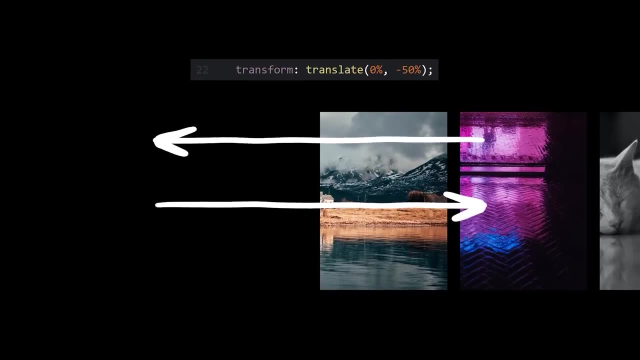 that has been slid Now. if we recall, earlier we used the translate property to shift our slider up by 50% of its height. Well, thanks to this value here we can perform a very similar manipulation in the left-right direction. For instance, if we set this value to negative 50%, our track moves. 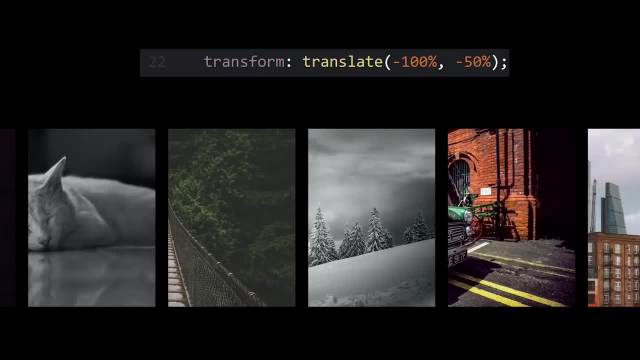 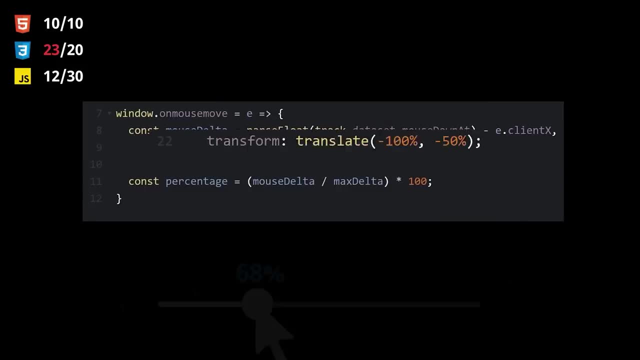 50% in the left direction. If we set it to negative 100%, our track has moved all the way to the right. Fortunately, since we just spent all that time calculating the percentage value of our magic slider, the next step is easy. We simply use this value to set the left-right percentage on our track. 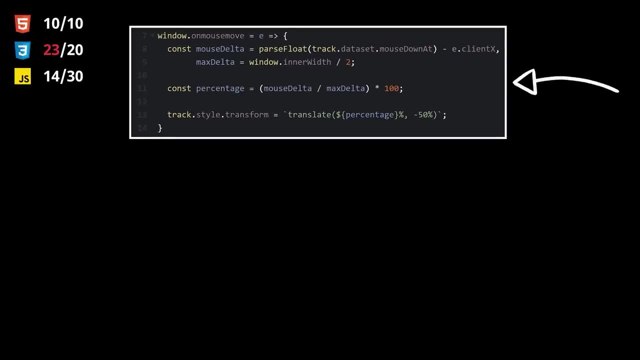 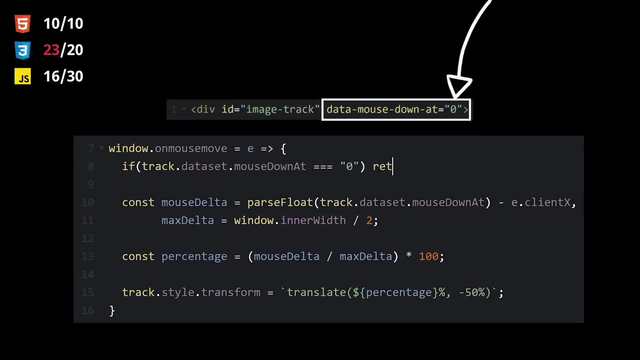 and… whoa, whoa, hang on. The mouse move. listener has no way of knowing when the mouse is actually down, So the track is moving before it's supposed to. Well, since I know the mouse down at position is zero before the mouse is pressed, we could just say that, if that's the case, return immediately. 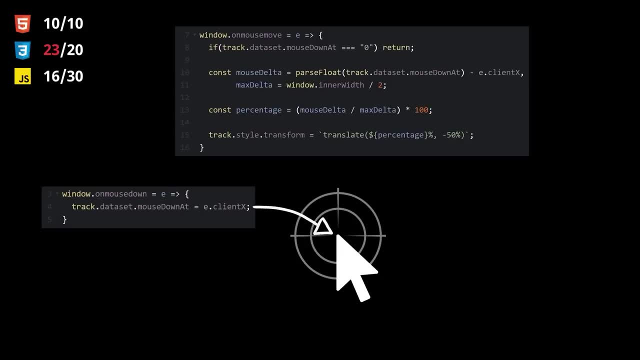 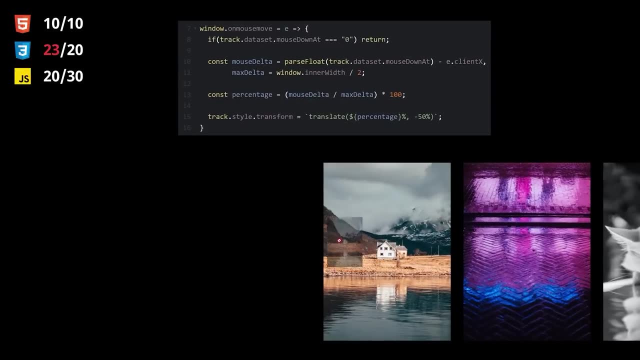 and skip the code that's telling the track to move. But as soon as the user clicks, the value will no longer be set to zero, So we'll have to set it back to zero when they release the mouse. Uh okay, So now when I click an image, it just drags it off the track. Stupid default behavior. 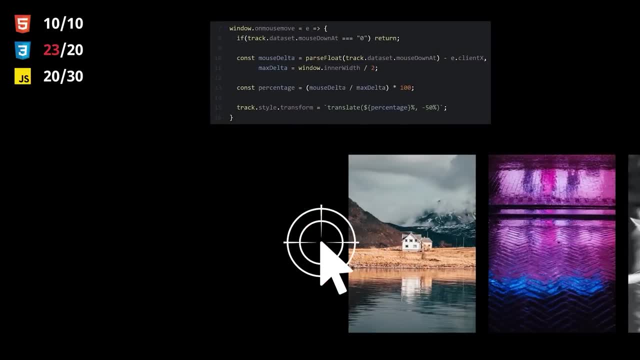 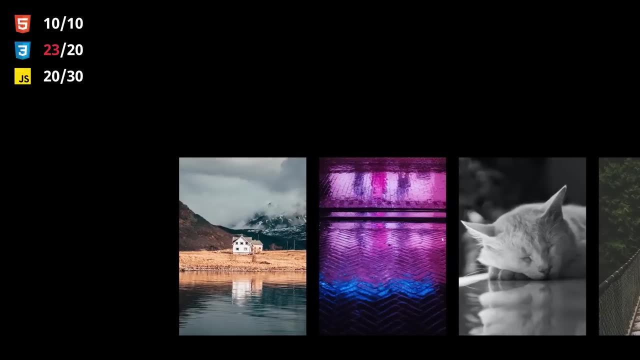 Fine, We'll just set draggable to false. Okay, no more weird dragging. but we're clearly going in the wrong direction here, so I guess we gotta flip the sign. Alright, looking good here. Wait, why is the position resetting when I try to drag a second time? Are you kidding? Since we're not, 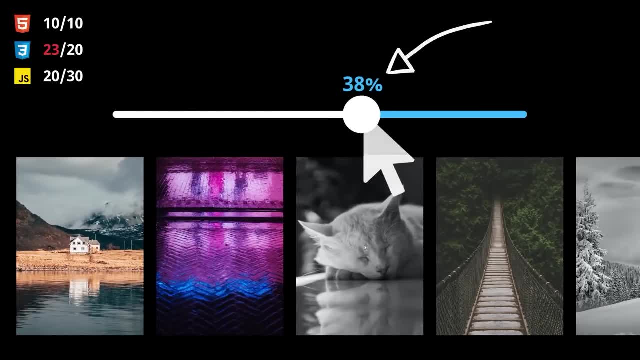 keeping track of how far we've dragged the slider, instead of continuing from where it was left off, it just resets back to zero. So we're not keeping track of how far we've dragged the slider. instead of continuing from where it was left off, it just resets back to zero. 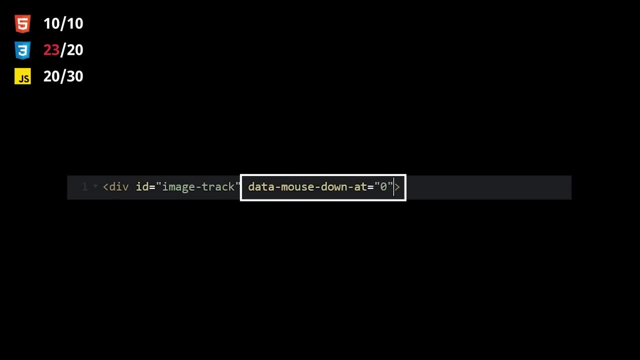 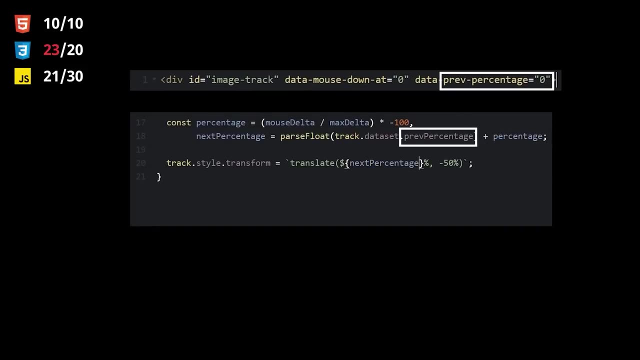 Fine, Okay, so just like we stored the mouse down position with the track, we're gonna have to store the percentage there too, I'm guessing. That way we can take the current percentage slid and add it to the last percentage to get the new percentage. 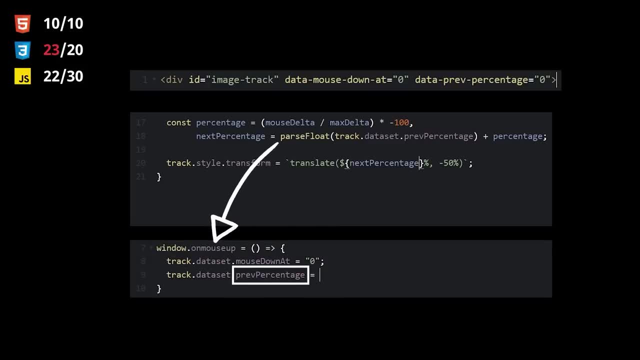 So we need to store this value every time they release the mouse. but how do we get that value from the mouse move listener. Okay. what if we constantly update the percentage here and then use it purely as a way to transfer the value between the two? 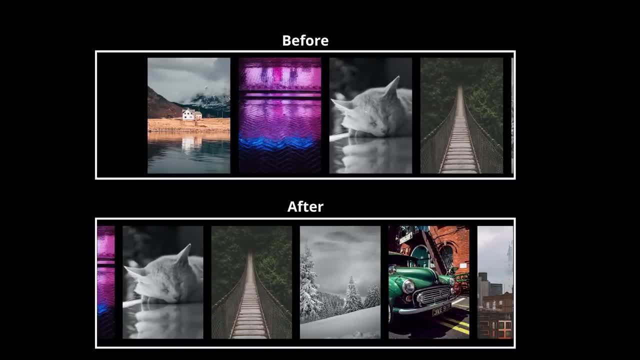 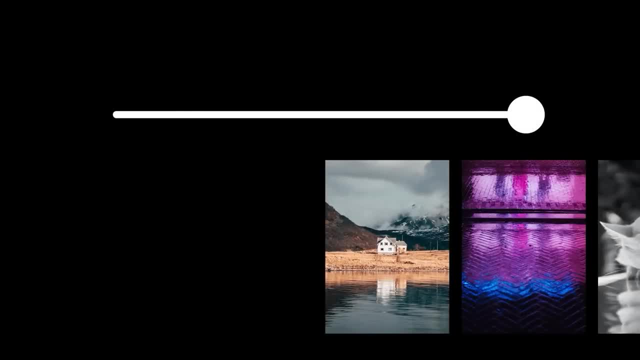 Aha, there we go. Now, when I click and drag a second time, it continues from where we left off, rather than resetting back to the default position of zero. Boy, we really got off in the weeds again there. What the heck just happened? Right, so our click and drag was technically 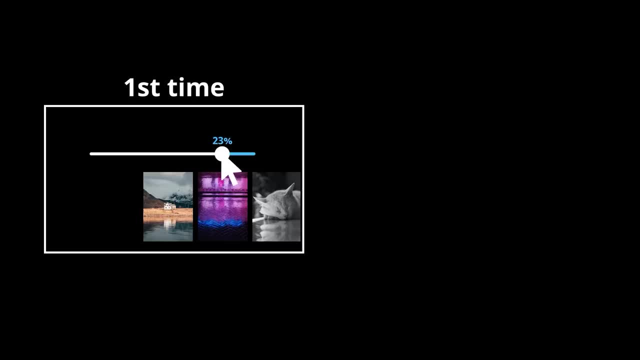 working, but only if it was the first time the user had ever moved the track. What we failed to account for was that the next time the user decides to click and drag, their progress wasn't stored anywhere, so the track had no way of knowing it should no longer start at zero.